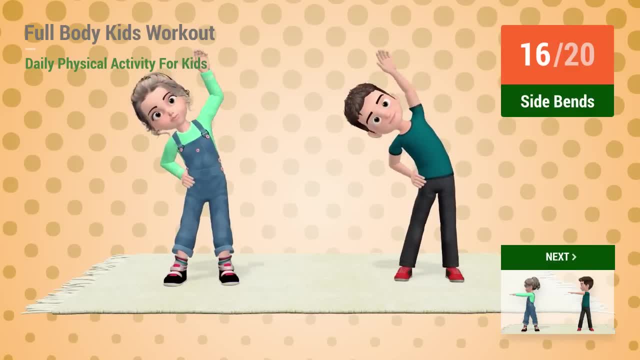 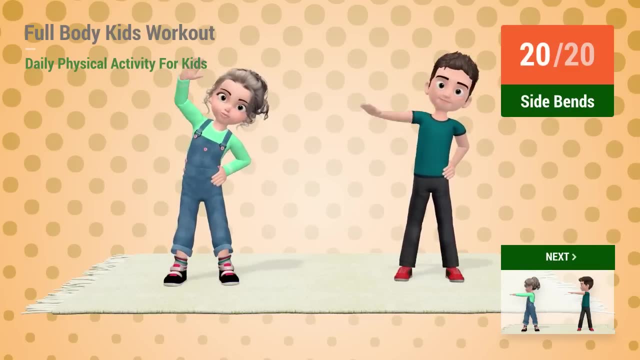 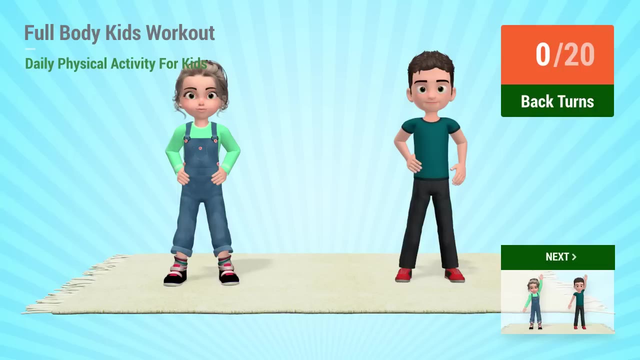 16,, 17,, 18,, 19,, 20.. Up next back turns in 5,, 4,, 3,, 2, 1. Go 1,, 2,, 3,, 4,, 5.. 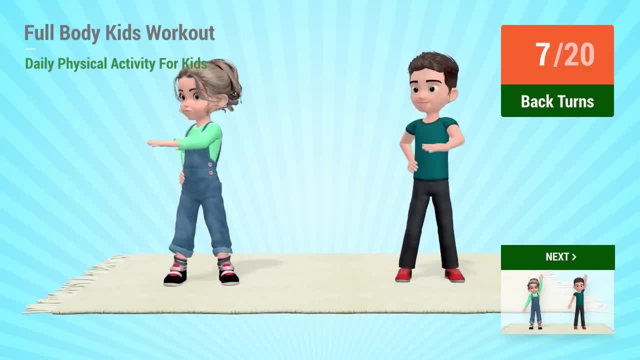 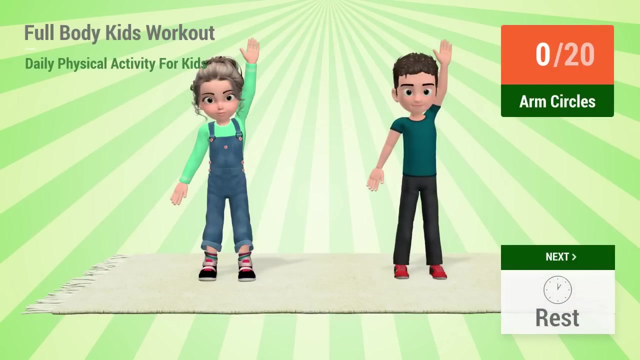 6,, 7,, 8,, 9,, 10,, 11,, 12,, 13,, 14,, 15,, 16,, 17,, 18,, 19, 20.. Up next arm circles In 5,, 4,, 3,, 2,, 1, go. 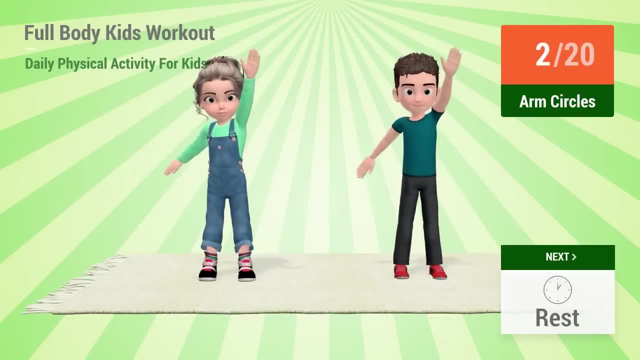 1,, 2,, 3,, 4,, 5,, 6,, 7,, 8,, 9,, 10,, 11,, 12,, 13,, 14,, 15,, 16,, 17,, 18,, 19, 20.. 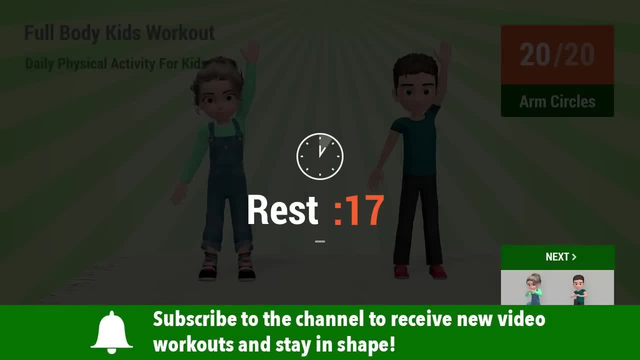 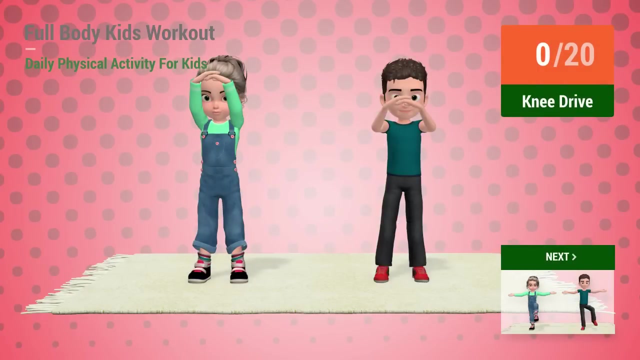 Rest Up next knee drive In 5,, 4,, 3,, 2,, 1, go 1,, 2,, 3,, 4,, 5,, 6,, 7,, 8,, 9,, 10,, 11,, 12,, 13,, 18,, 19,, 20.. 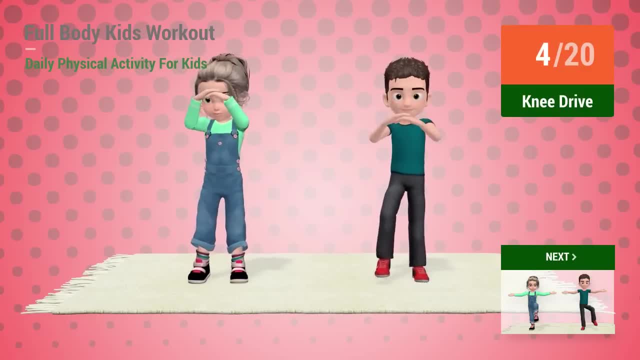 Up next knee. drive In 5,, 4,, 3,, 2,, 1, go 1,, 2,, 3,, 4,, 5,, 6,, 7,, 8,, 9,, 10,, 11,, 12,, 13,, 14,, 15,, 16,, 17,, 18,, 19, 20.. 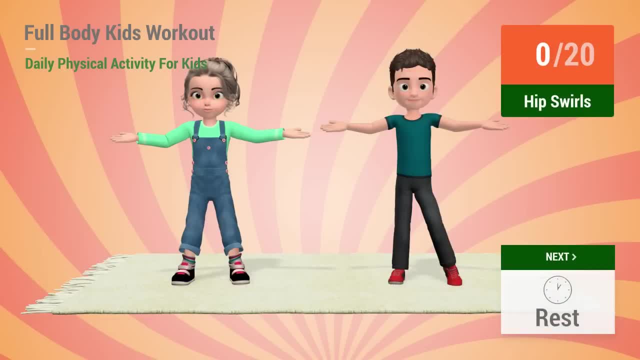 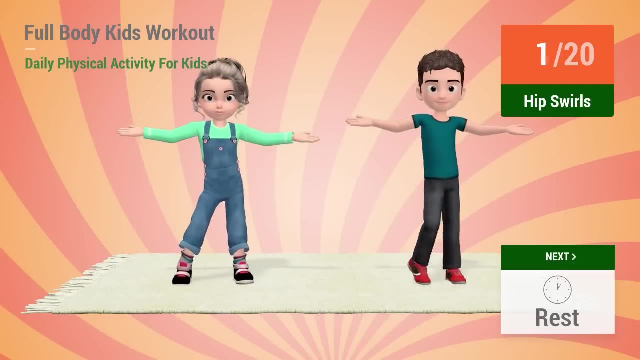 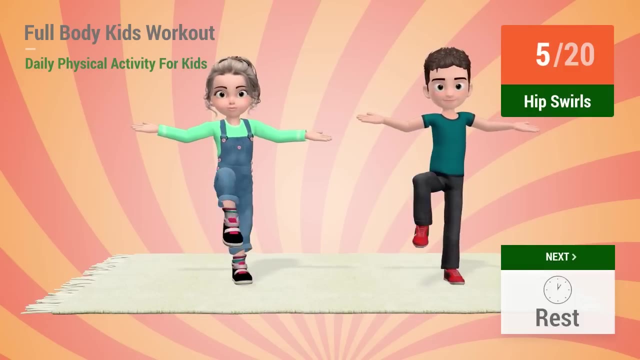 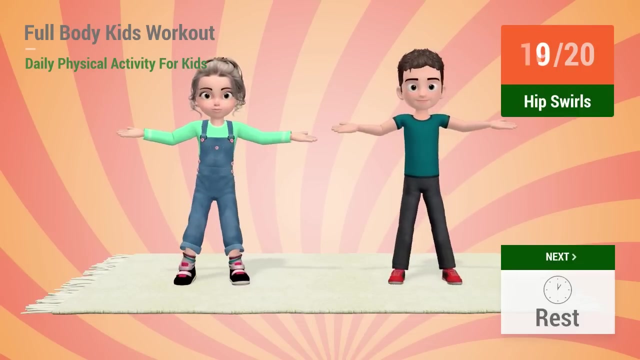 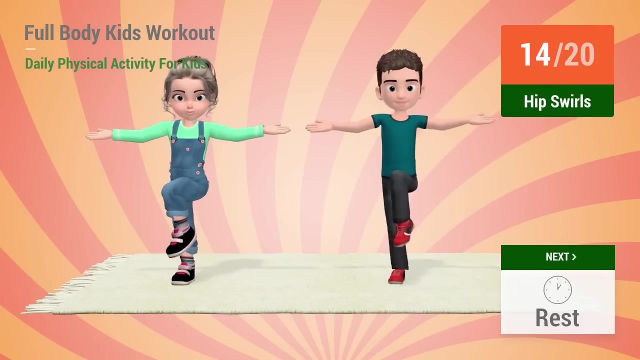 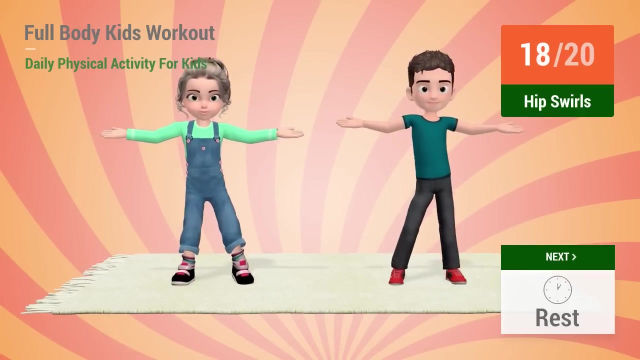 Up next hip swirls In 5,, 4,, 3,, 2,, 1, go 1,, 2,, 3,, 4,, 5,, 6,, 7,, 8,, 9,, 10,, 11,, 12,, 13,, 14,, 15,, 16,, 17,, 18,, 19,, 20.. 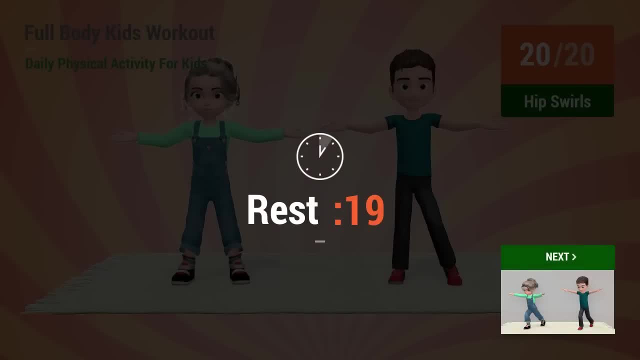 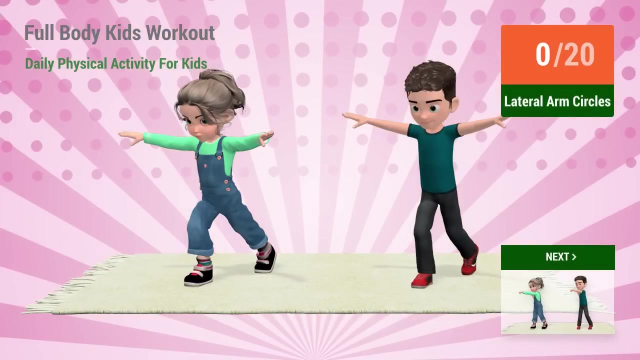 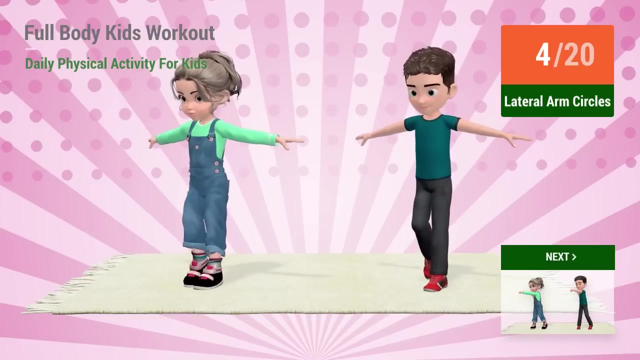 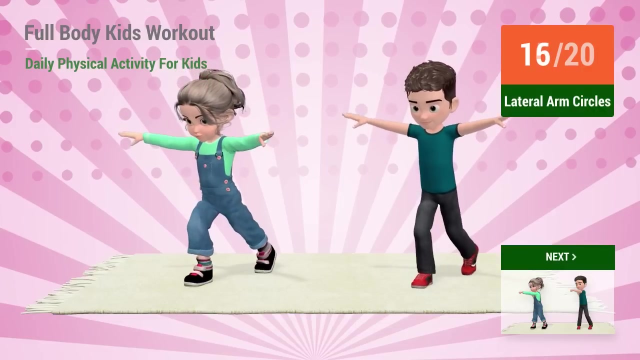 20.. Rest time Up next: lateral arm circles In 5,, 4,, 3,, 2,, 1, go 2, 1, go 1,, 2,, 3,, 4,, 5,, 6,, 7,, 8,, 9,, 10,, 11,, 12,, 13,, 14,, 15,, 16,, 17,, 18,, 19,, 20.. 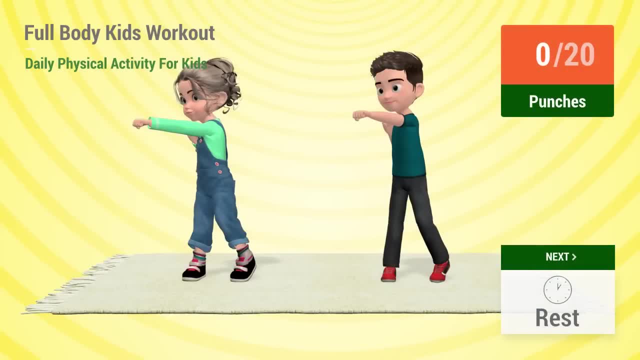 Up next Punches in 5,, 4,, 3,, 2,, 1, go 1,, 2,, 3,, 4,, 5,, 6,, 7,, 8,, 9,, 10,, 11,, 12,, 13,, 14,, 15,, 16,, 17,, 18,, 19,, 20.. 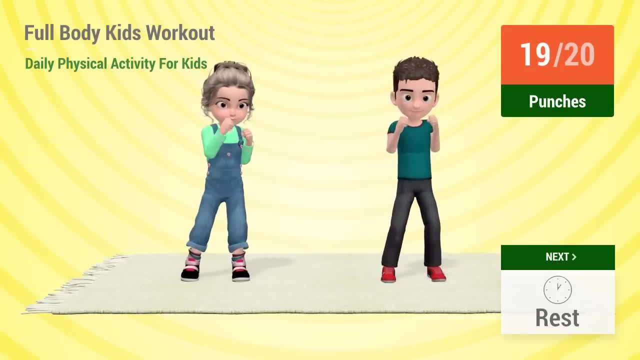 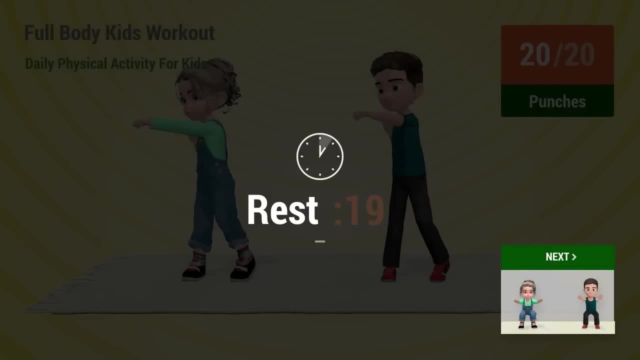 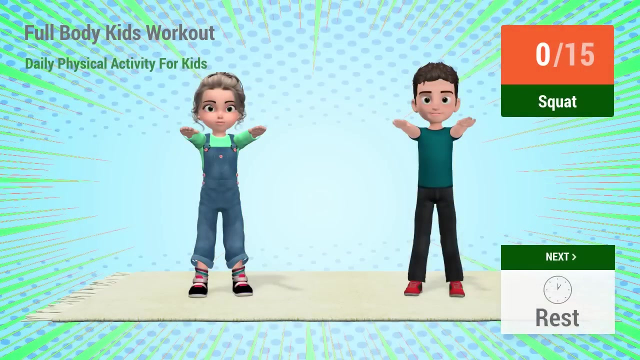 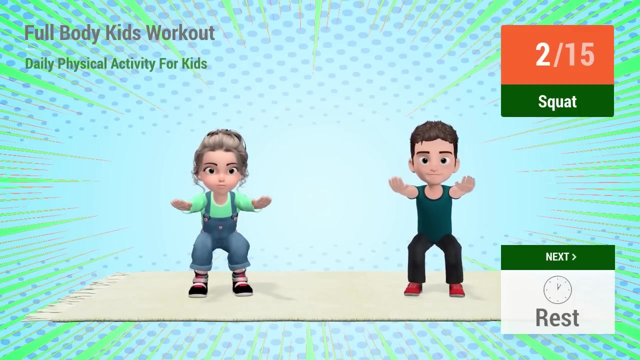 Rest time. Up next Squat in 5,, 4,, 3,, 2,, 1, go 1,, 2,, 3,, 4,, 5,, 6,, 7,, 8,, 9,, 10,, 11,, 12,, 13,, 14,, 15,, 16,, 18,, 19,, 20.. 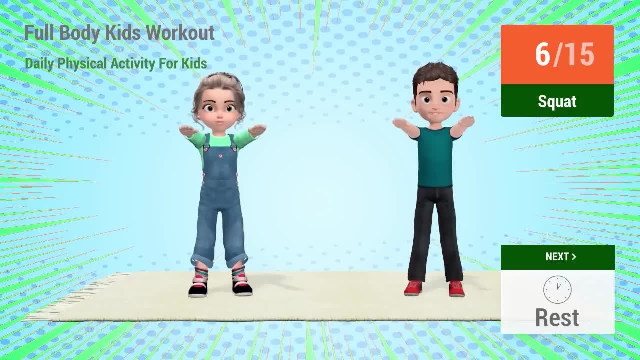 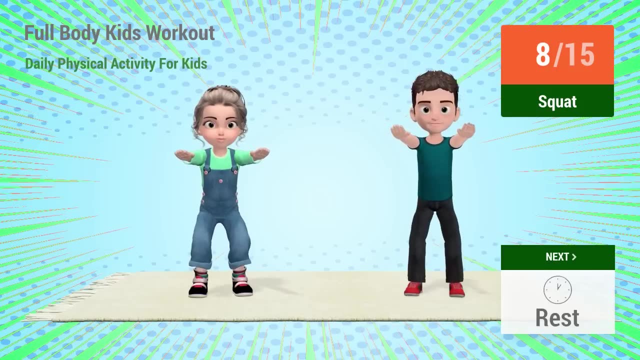 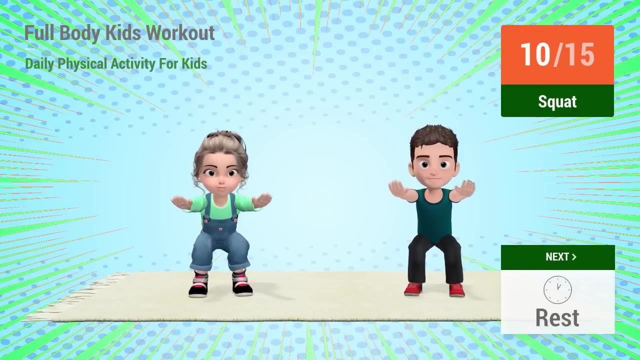 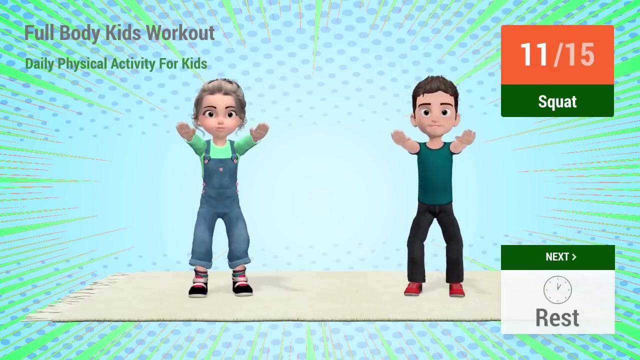 6,, 7,, 8,, 9,, 10,, 11,, 12,, 13,, 14,, 15,, 16,, 17,, 18,, 19,, 20. 13., 14, 15. 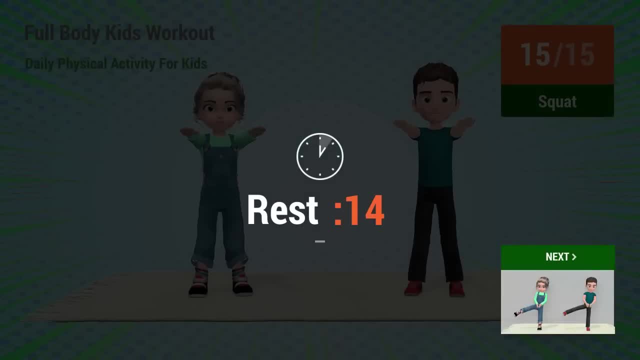 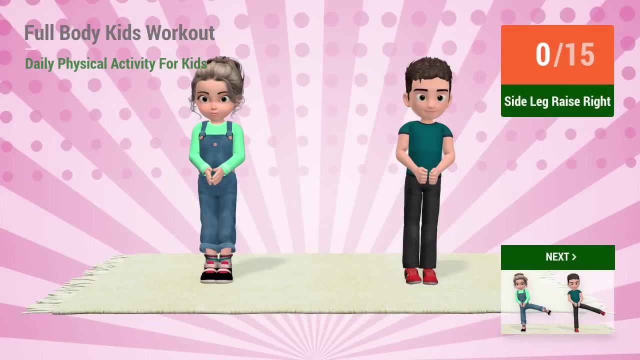 Rest time. Up next Side leg raises in 5,, 4,, 3, 2, 1, go 1, 2, 3, 4, 5, 6, 7, 8, 9, 10, 11, 12. 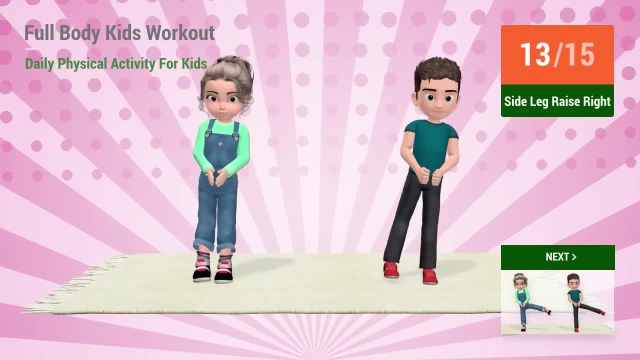 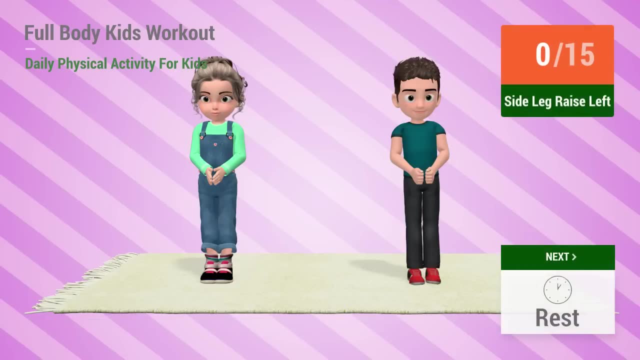 13, 14, 15. Up next Side leg raises in 5,, 4,, 3, 2, 1, go 1, 2, 3, 4, 5, 6, 7, 8, 9, 10, 11. 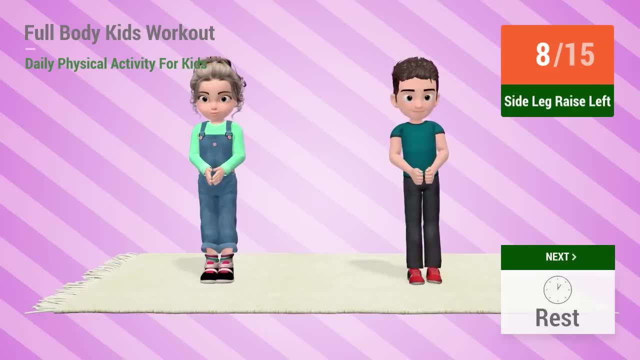 12, 13, 14, 15. Rest time: Up next Side leg raises in 5,, 4,, 3, 2, 1, go 1, 2, 3, 3, 4, 5, 6, 7. 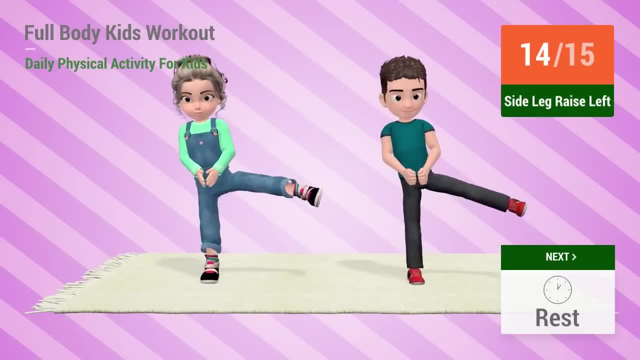 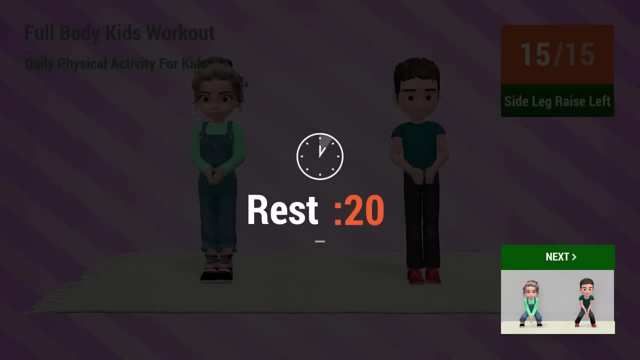 8, 9, 10, 11, 12, 13, 14, 15, 16, 17, 18, 19, 20, 23, 24, 25, 26, 27, 28, 29, 30, 33, 34, 35, 36, 37. 38, 38, 39, 40, 41, 42, 43, 44, 45, 46, 47, 48, 49, 50, 51, 52, 53, 54, 55, 56, 57, 58, 59, 60, 61, 62. 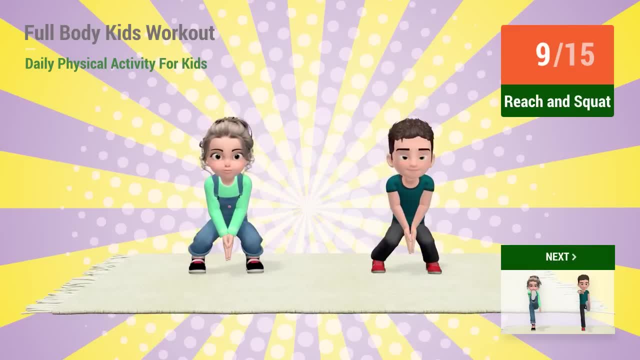 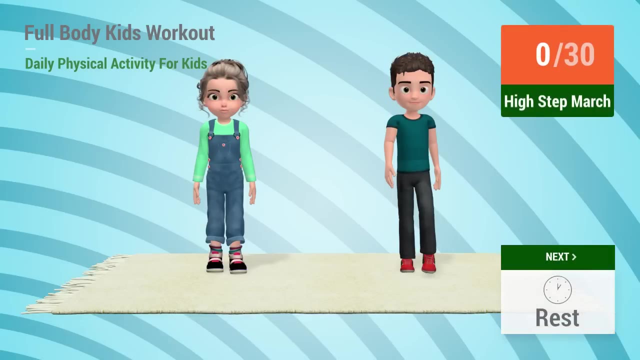 63, 64, 65, 66, 67, 68, 69, 70, 71, 72, 73, 74, 75, 76, 77, 78, 79, 80, 81, 82, 83, 83, 84, 85, 86, 87. 88, 89, 90, 91, 92, 93, 94, 95, 96, 97, 97, 98, 99, 100, 100, 100, 11, 11, 12, 13, 14, 15, 16, 17, 18, 19. 20, 21, 22, 23, 24, 25, 26, 27, 28, 29, 30, Rest Time: 26, 27, 28, 29, 30, 31, 32, 33, 34, 35, 36, 37, 38, 39. 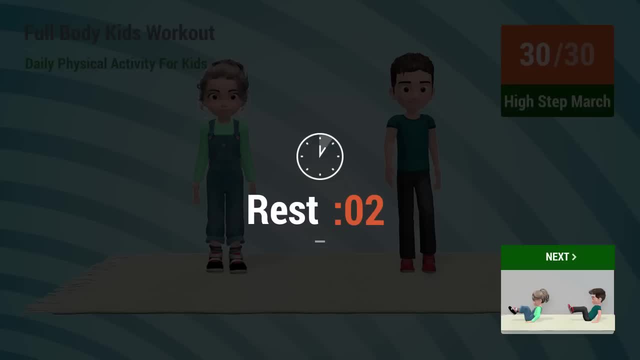 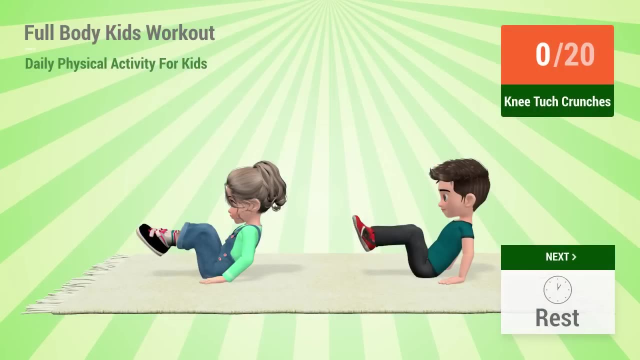 40, 41, 42, 43, 44, 45, 46, 47, 48, 49, 50, 51, 52, 53, 53, 54, 55, 56, 57, 58, 59, 60, 61, 62, 63, 64. 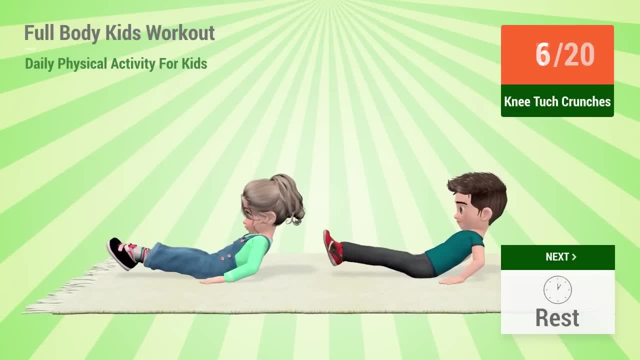 65, 66, 67, 68, 69, 70, 71, 72, 73, 74, 75, 76, 77, 78, 79, 80, 81, 82, 83, 83, 84, 85, 86, 87, 88, 89. 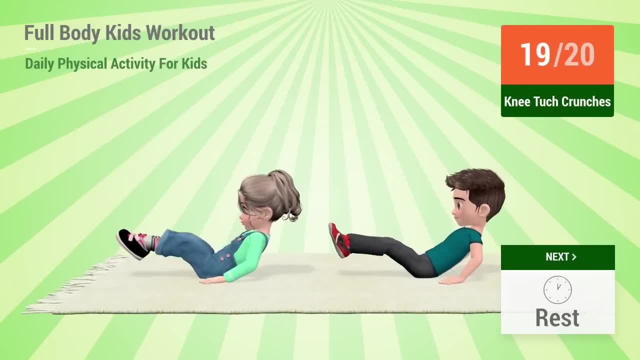 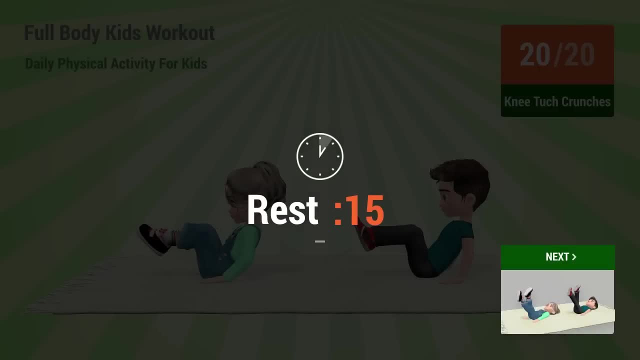 90, 91, 92, 93, 94, 95, 96, 97, 98, 99, 100, 100, 11, 12, 13, 14, 15, 16, 17, 18, 19, 20, Rest Time 20, 23, 24. 25, 26, 27, 28, 29, 30, 31, 32, 33, 34, 35, 36, 37, 38, 38, 39, 40, 41, 42, 43, 44, 45, 46, 47, 48, 49. 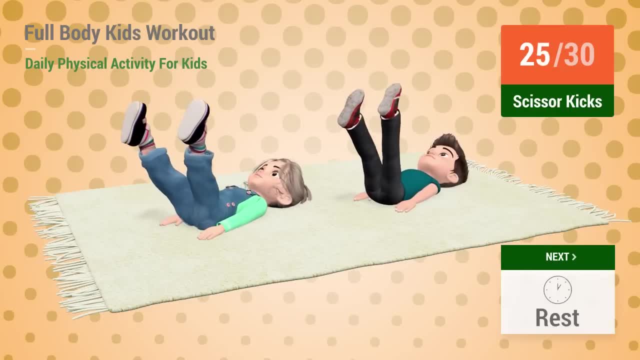 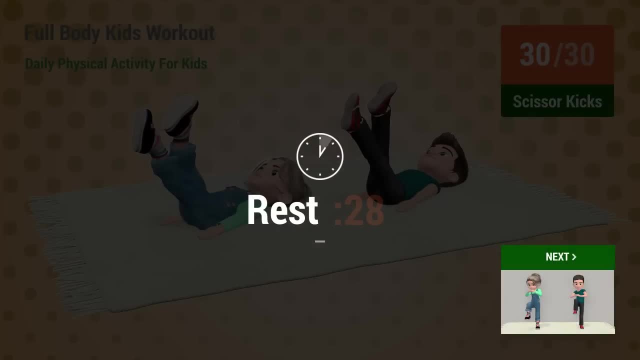 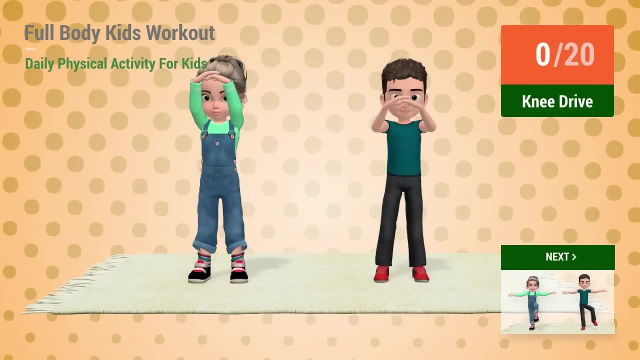 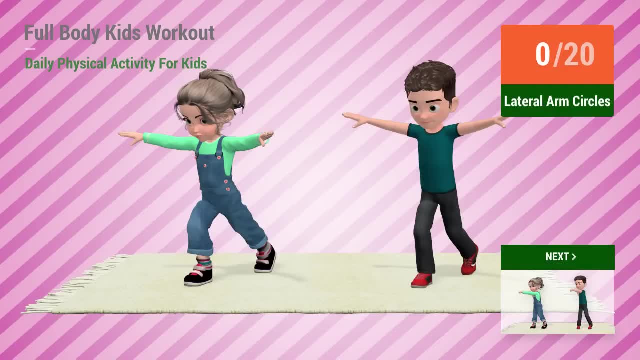 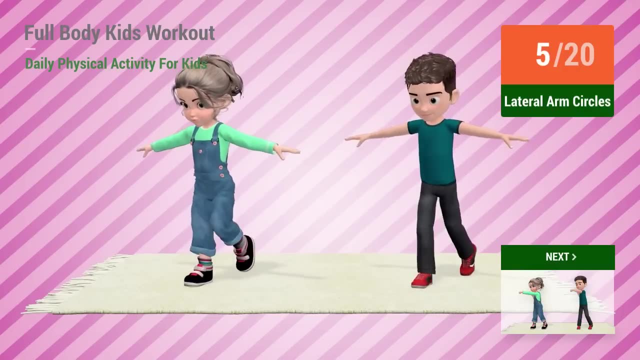 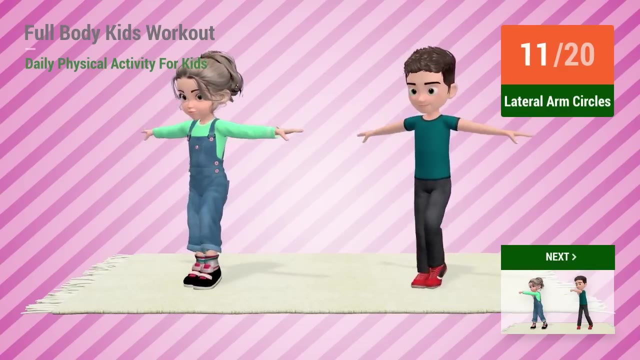 27, 28, 29, 19, 18 go. 1, 2, 3, 4, 5, 6, 7, 8, 9, 10, 11, 12, 13, 14, 15, 16, 17, 18, 19, 20 up next. 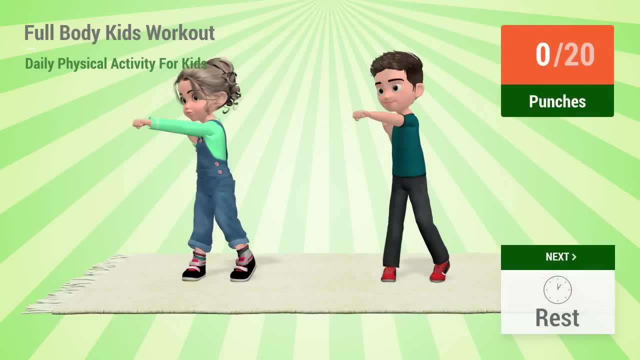 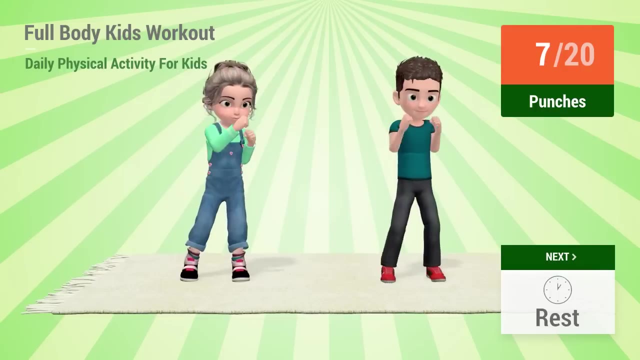 punches in 5, 4, 3, 2, 1 go. 1, 2, 3, 4, 5, 6, 7, 8, 9, 10, 11, 12, 13, 14, 15, 16. up. next punches in 5, 4, 3, 2, 1 go. 1, 2, 3, 4, 5, 6, 7, 8, 9, 10, 11, 12, 13, 14, 15, 16, 17, 18. 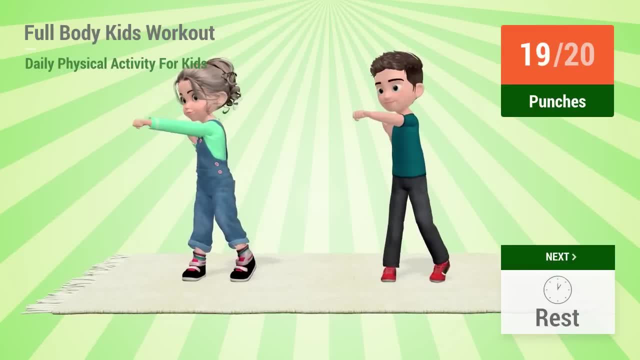 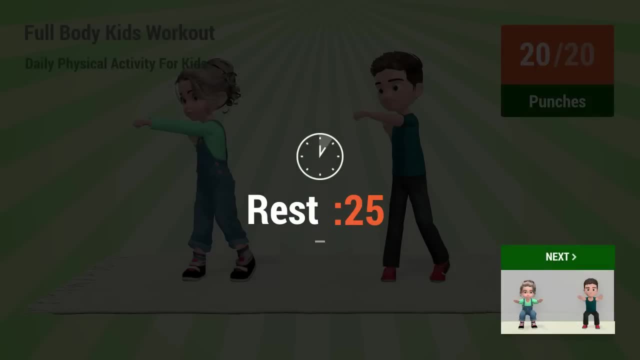 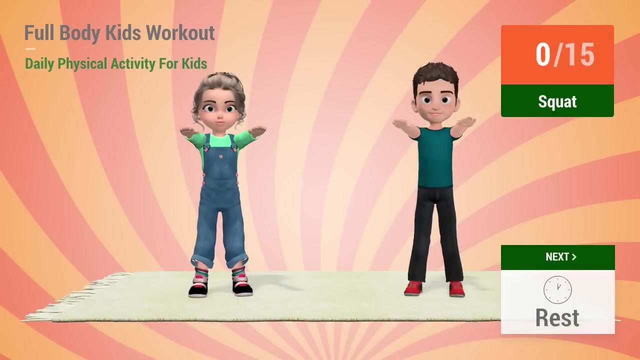 17, 18, 19, 20 rest time. up next squat in 5, 4, 3, 2, 1 go. 1, 2, 3 4 go. 1 go. 1, 2, 3 go. 1 go, 1, 3, 2 go. 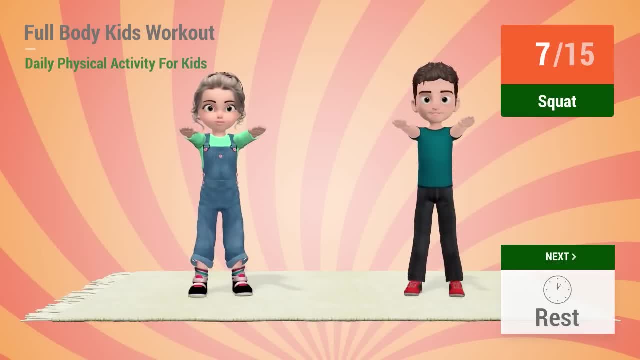 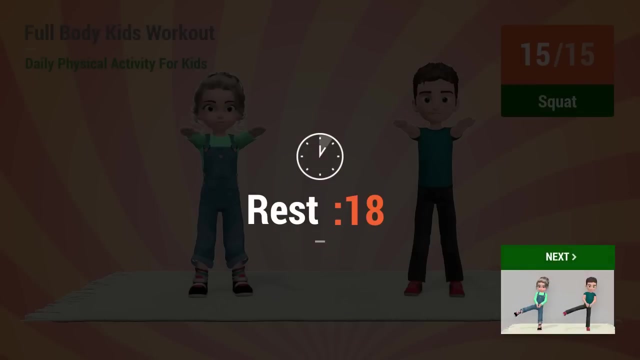 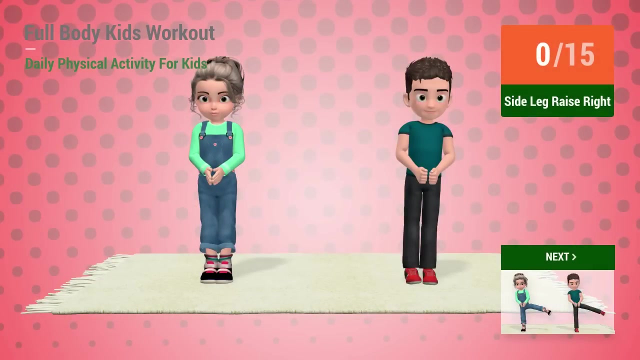 bye. 6, 7 A, 9, 10, 11, 12, 13, 14, 15. rest time up. next side leg raises in 5, 4, 3, 2, 1 go 1, 2, 3, 4, 5, 6. 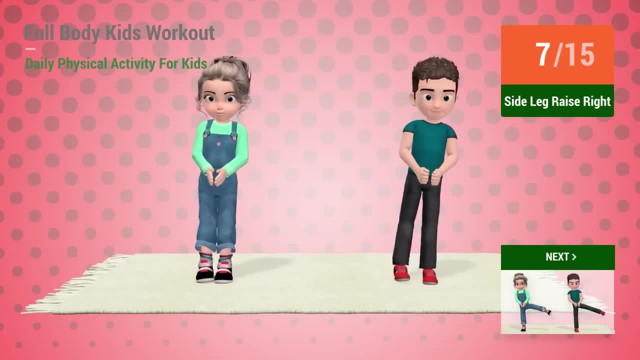 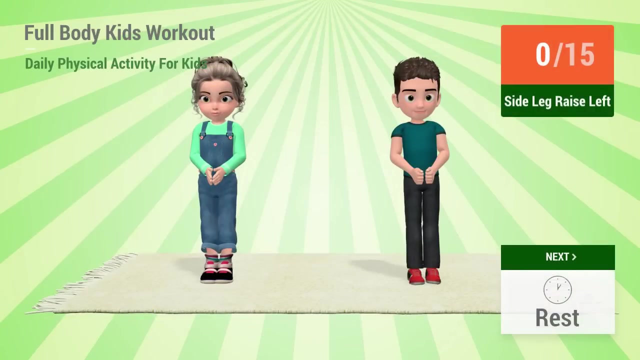 7, 8, 9, 10, 11, 12, 13, 14, 15, 7, 8, 9, 10, 11, 12, 13, 14, 15. up. next side leg raises in 5, 4, 3, 2. 1. go 1, 2, 3, 4, 5, 6. 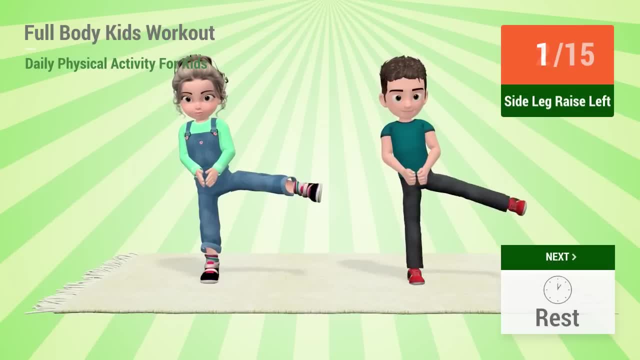 1, 2, 3, 4, 5, 6, 7, 8, 9, 10, 11, 12, 13, 14, 15. up. next side leg raises in 5, 4, 3, 2, 1 go. 1, 2, 3, 4, 5, 6, 7, 8, 9, 10, 11, 12, 13, 15. up next side leg raises in: 5, 4, 3, 2, 1 go 1, 2, 3, 2, 1 go 1 2, 5, 6, 8, 8, 9, 10, 11, 12, 13, 14, 15 rest time. 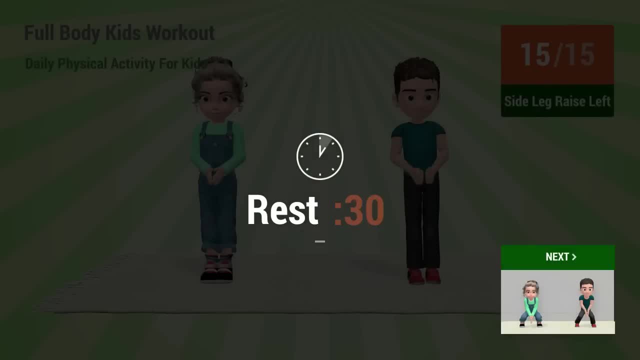 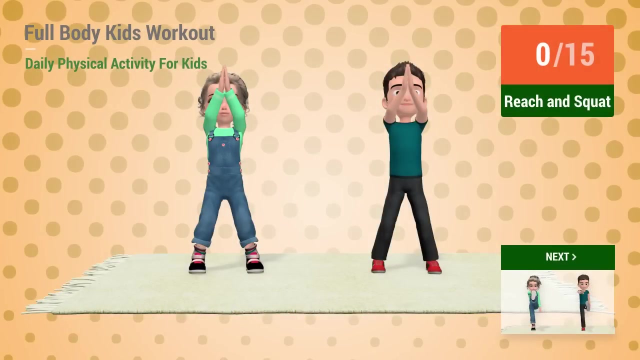 8, 8, 9, 9, 10, 11, 12, 13, 14, 15. rest time up next. reach and squat in five, four, three, two, one. go one, two, three, four, five, six, seven, eight, nine, ten, 11, 12, 13, 14, 15 up next. 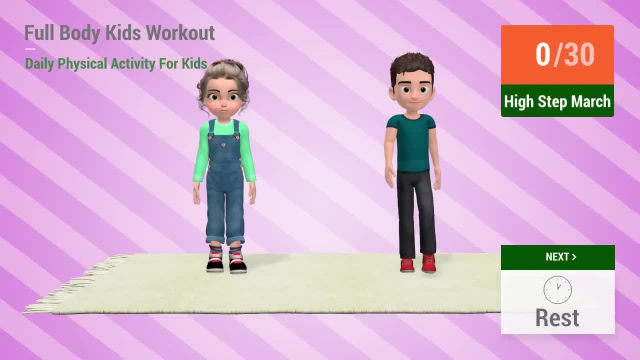 high step. march in 5, 4, 3, 2, 1 go 1, 2, 0, three, four, five, six, seven, eight, nine, ten, eleven, twelve, thirteen, fourteen, fifteen, sixteen, seventeen, eighteen, nineteen, twenty, twenty-one, twenty-two, twenty-three, twenty-four. 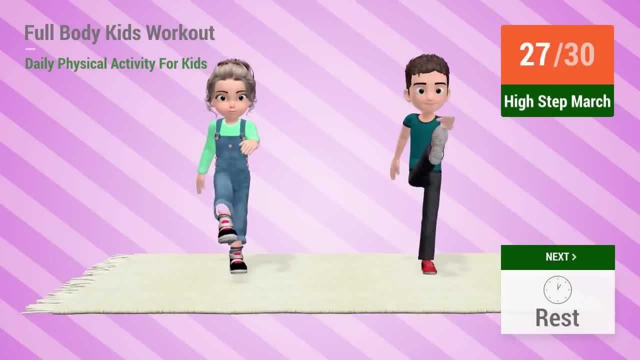 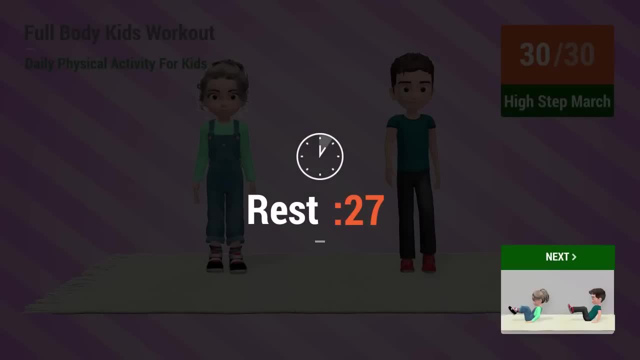 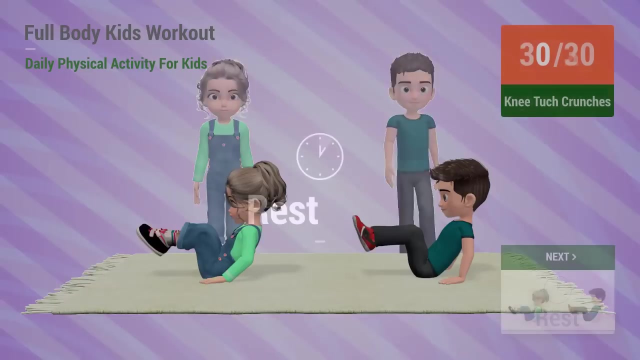 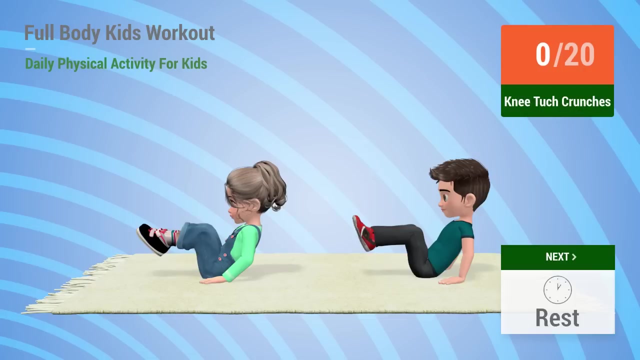 twenty-five, twenty-six, twenty-seven, twenty-eight, twenty-nine, thirty, Rest time. Up next knee tuck crunches In five, four, three, two. one go. One, two, three, four, five, six, seven, eight, nine, ten, eleven, twelve, thirteen. 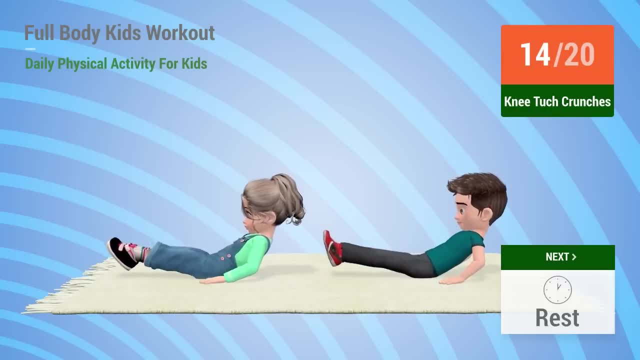 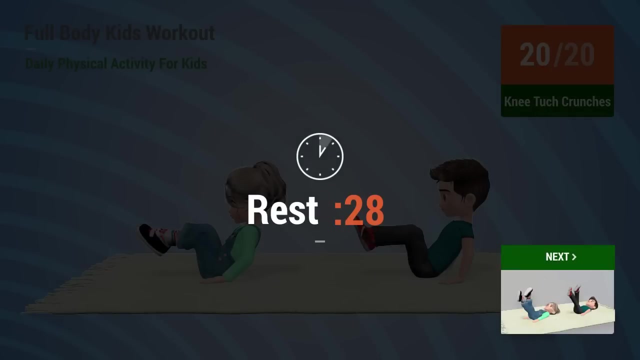 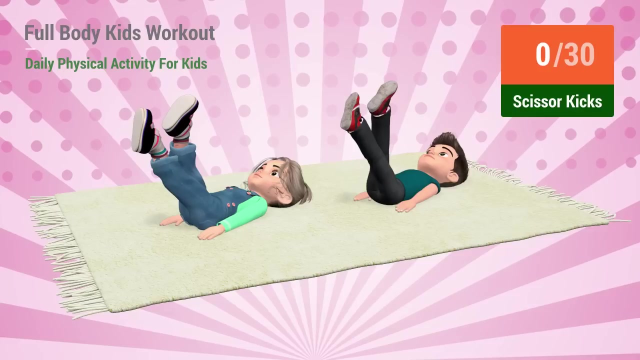 fourteen, fifteen, 15,, 16,, 17,, 18,, 19,, 20.. Rest time: Up next, scissor kicks in 5,, 4,, 3,, 2, 1.. Go 1, 2,, 3,, 4,, 5,, 6,, 7,, 8,, 9,, 10.. 11,, 12,, 13,, 14,, 15,, 16,, 17,, 18,, 19,, 20,, 21,, 22,, 23,, 24,, 25,, 26,, 27,, 28,, 29,, 30..